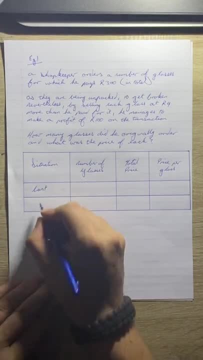 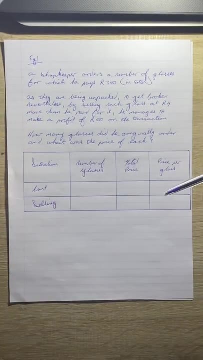 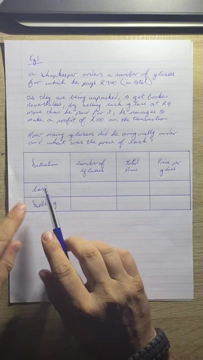 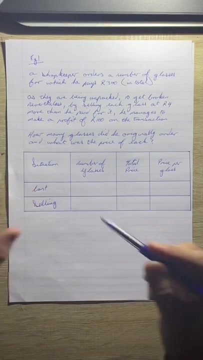 and the other situation will be selling- Okay, the cost would be buying the glasses and the selling would be the sale of them. Right now, let's have a look at this situation. for the cost, Okay, the number of glasses, well, that's what we don't know. So, always with these word problems, something that you don't know, you. 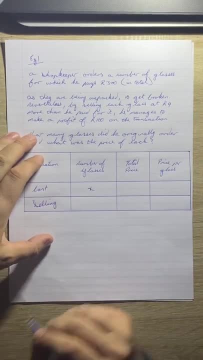 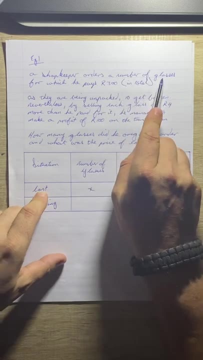 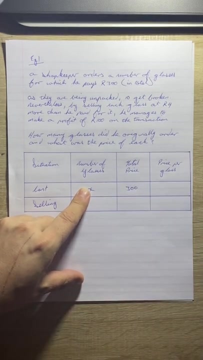 always let be x. Okay, now, what was the total price Of the cost? Well, they told us, here a shopkeeper orders the number of glasses, which we said was x, for which he pays 300 rand. So the total price for that is 300.. Then, in order to work out the price, 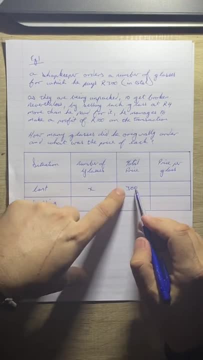 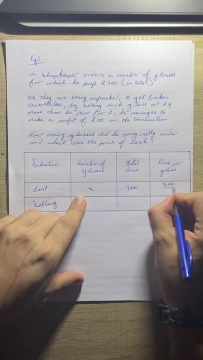 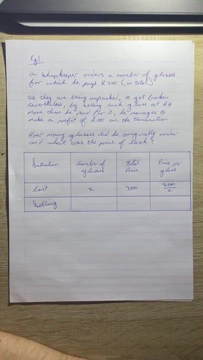 per glass. what we have to do is we have to take our total that we paid divided by the total number of glasses. So that would be 300 divided by x, and that will give us the price per glass. All right, now let's have a look at the selling. Now the selling: something happens. It says here: 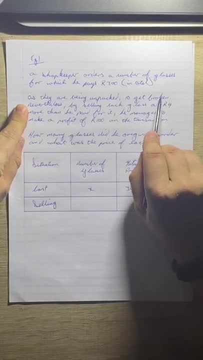 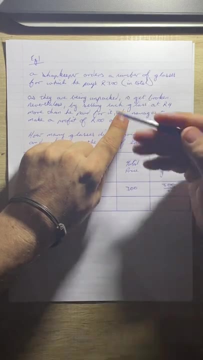 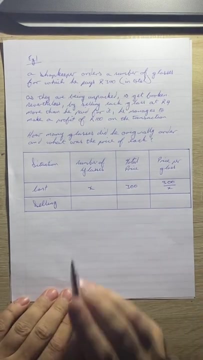 as they are being unpacked, 10 get broken Nevertheless by selling each glass. So I'm going to stop there. So 10 were broken, So you had 10 less to sell. So if you originally had x amount, So how many is he selling now? It's going to be the original amount minus 10.. Those 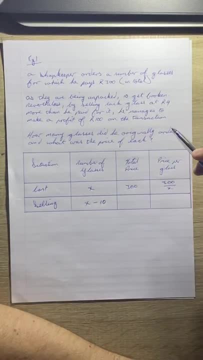 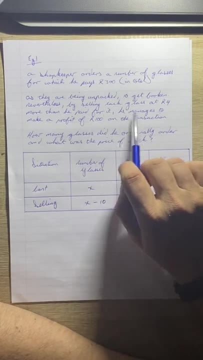 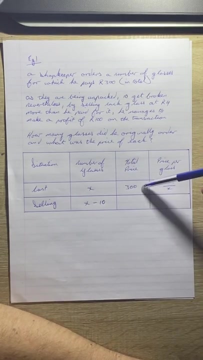 are the ones that were broken. Okay, It goes on to say here, selling each glass at four and more than he paid for it, He manages to make a profit of 100 rand on the transaction. Now, if he bought total these glasses for 300. 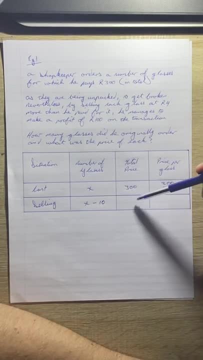 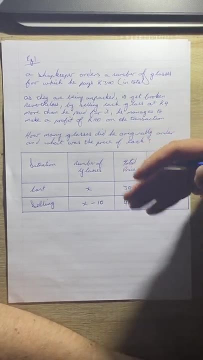 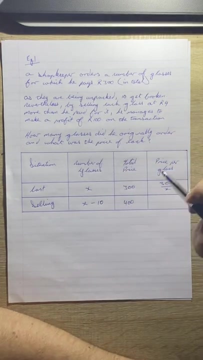 and he made a profit of 100. that means that he sold all of these glasses for 400 rand. Okay, because you know how to work out profit. It's your selling minus Your cost, Okay, In other words, 400 minus the 300, to give us 100 grand profit. Okay, Now the 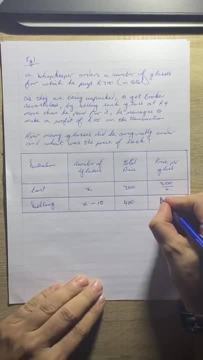 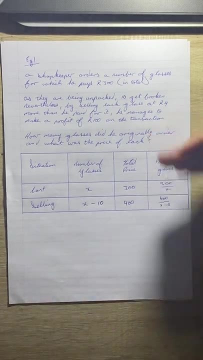 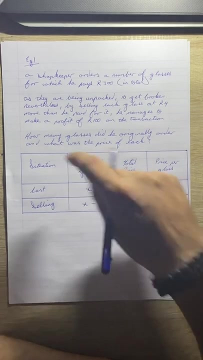 price per glass. Well, we've got the price, the total price, there, and we've got the total number of glasses, which is x minus 10.. Okay, So we've built up our little table. Now what we need to do is we need to make an equation in order to solve for what x is. Okay, Now there's 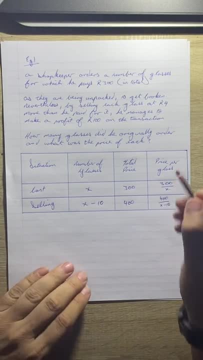 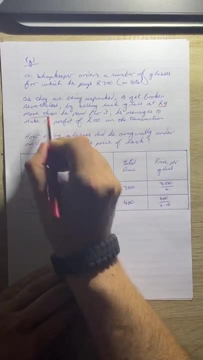 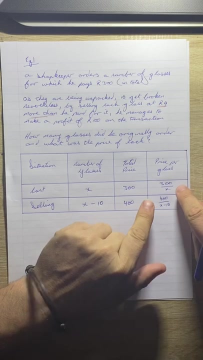 one little bit of information that we haven't used, and it's this: by selling each glass at four rand more, Okay, We haven't used that bit of information in our table. Now, how would that work with what we've got here? Now, just remember, we've got the price per glass for the cost, and we 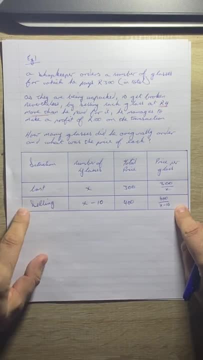 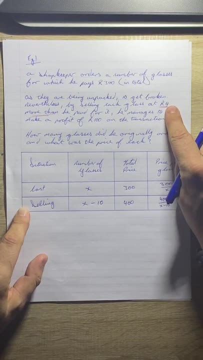 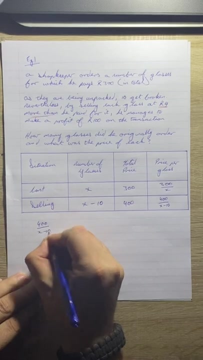 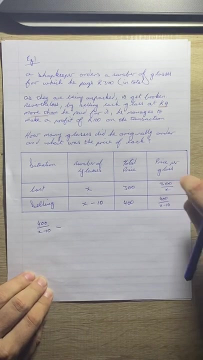 have the price per glass for the selling. Now, if we take the selling price per glass minus the cost, that should be four rand. Okay, So that's what I'm going to do. I'm going to take the 400 over x minus 10, which is our selling price per glass, and I'm going to subtract the cost price. 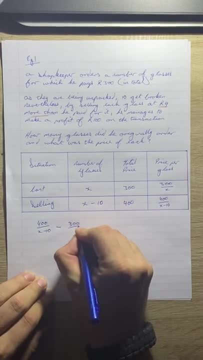 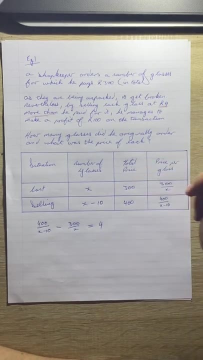 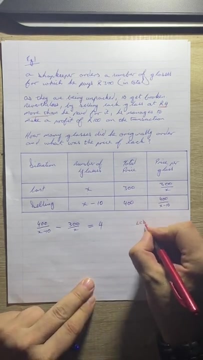 per glass, And that should be equal to four rand. Okay, So what I'm going to do now is I'm just going to solve for this. This is an equation that you guys have been working with The last few weeks. you find an LCD, and our LCD in this case is x x minus 10.. So I'm going to 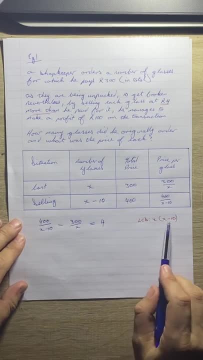 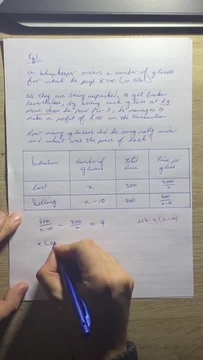 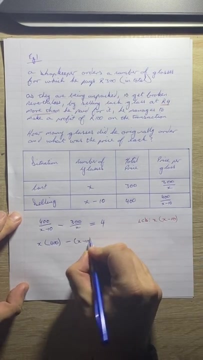 multiply everything by that. If I multiply this by LCD, the x minus 10 will cancel with x minus 10 and you're just left with x multiplied by that 400 minus. multiply this by LCD. What are we left with? We're left with x minus 10 multiplied by 300.. And on this side we're just. 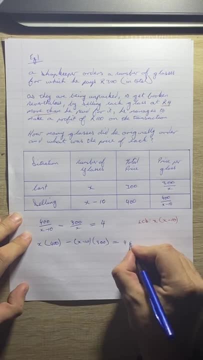 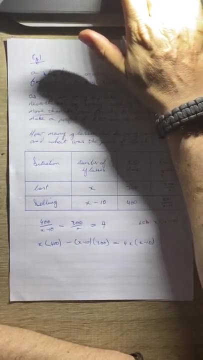 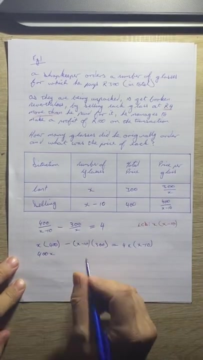 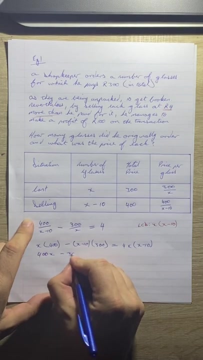 left with four multiplied by x, multiplied by x minus 10.. Okay, What we can do now is we can just simplify that by multiplying out, So that will give us 400 x. This here I'm going to do one time. So we've got the minus 300 times x, gives us minus 300 x, Then minus 300 times minus 10. 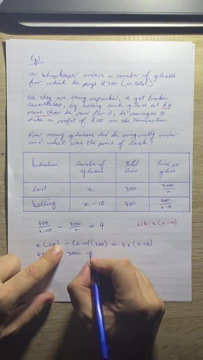 gives us minus 300 x, And then minus 300 times minus 10 gives us minus 300 x, And then minus 3 plus 3000.. Because the minus and the minus gives us the plus. So we get plus 3000 equals. 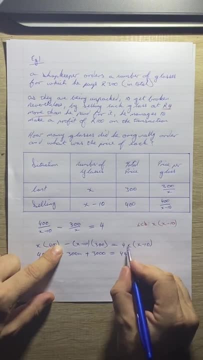 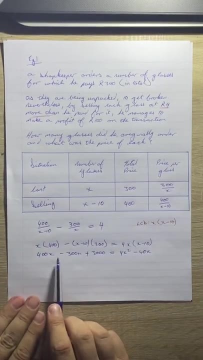 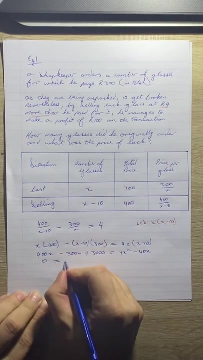 multiply this in here we get 4 x squared, minus 40 x. Okay, So what I think I'm going to do here, grade 11s, is I'm going to take everything to the right hand side and set this equal to zero. All right, So we get zero is equal to 4 x squared. Then we've got minus 40.. 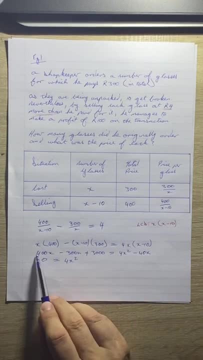 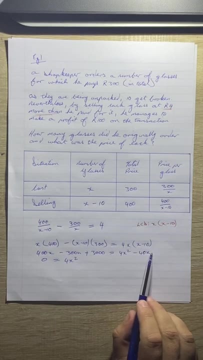 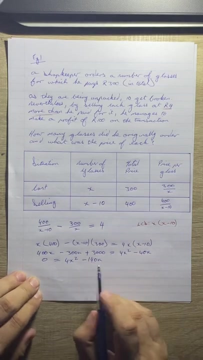 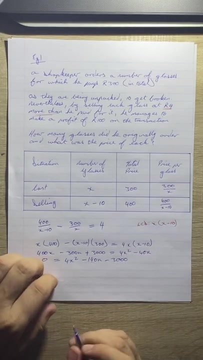 Minus 400 plus 300. Because I'm taking everything to the other side And we get minus 140 x, And then all we've got is this constant. Take it to the other side and it becomes minus 3000.. Okay, What I can do now is I can divide 3 by 4 to make our lives a little bit easier, And we get. 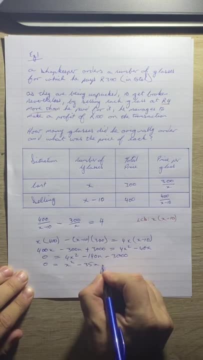 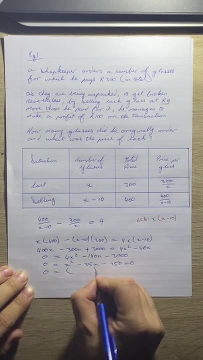 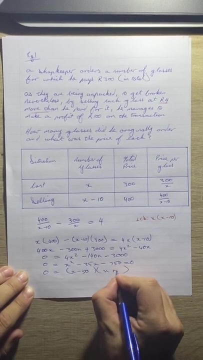 x squared minus 400 x, And then we get minus 400 x, And then we get minus 400 x, And then we get x squared minus 35. x minus 750 equals to zero. You can factorize this And we get x minus 50, x plus 15.. Then I can solve and we get: x is equal to 50 or x is equal to minus. 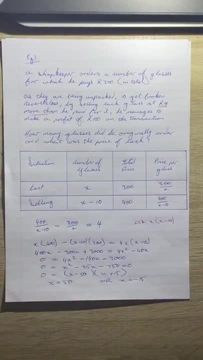 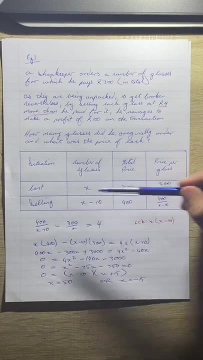 15.. Now what we've got to do is we've got to interpret our answers here and see what we've got. Remember, your x is the number of glasses that you bought. Okay, So, yes, it makes sense to buy 50 glasses. It doesn't. 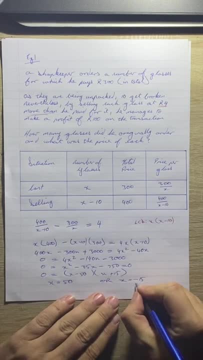 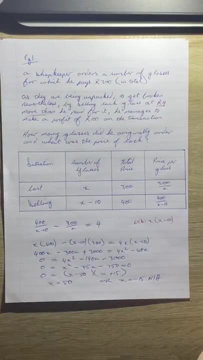 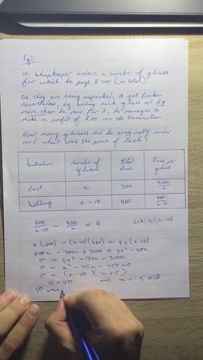 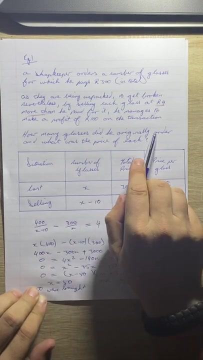 make sense to buy negative 15 glasses. So this answer here is not applicable. That one doesn't fit with our answer here. So therefore, 50 glasses were bought. Okay, That was this. How many glasses did he originally order Then? what was the price of?